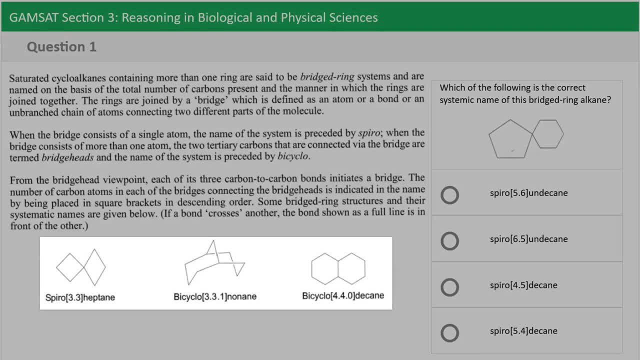 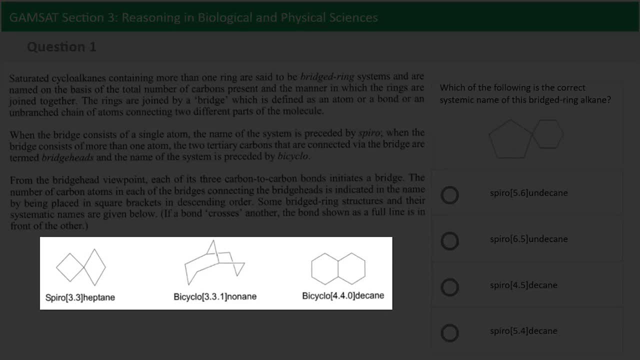 laid out there for you, but a quicker way might be to recognize the fact that some examples have already been provided. You know, I see there are other visual depictions of molecules that are already named, and perhaps what I can do is work backwards and figure out how to match up my picture. 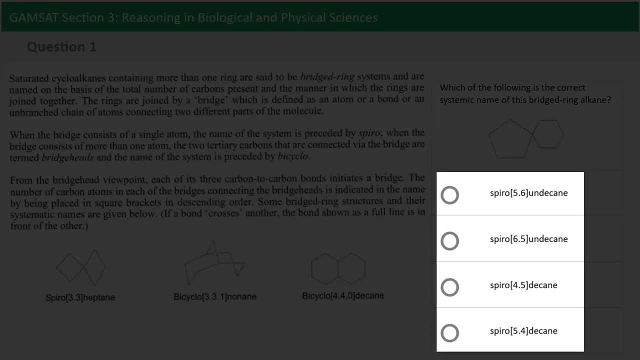 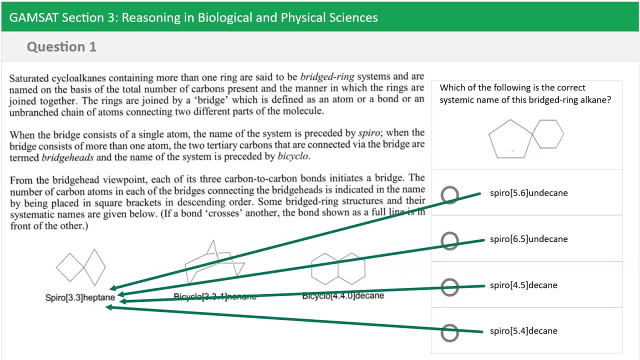 to one of the answer options. I'm going to use the answer options to guide me. It looks like it's directing me towards the first molecule here, which is called spiro, and in the brackets, 3,3-heptane, And I can tell just by looking at our molecule. 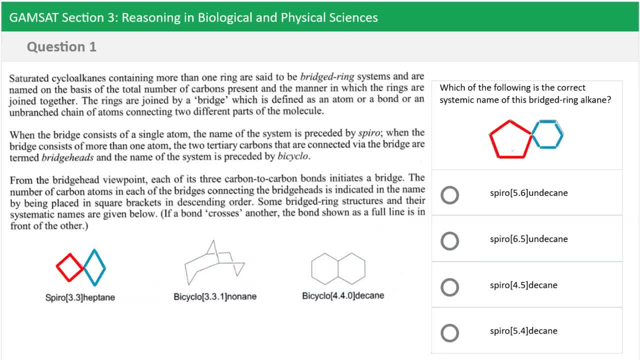 that there are some similarities. There are two ring structures which are connected by. it looks like one point. Okay, now, the fact that all of the options start off with spiro means that we don't need to prove that the molecule that we have is indeed named spiro. 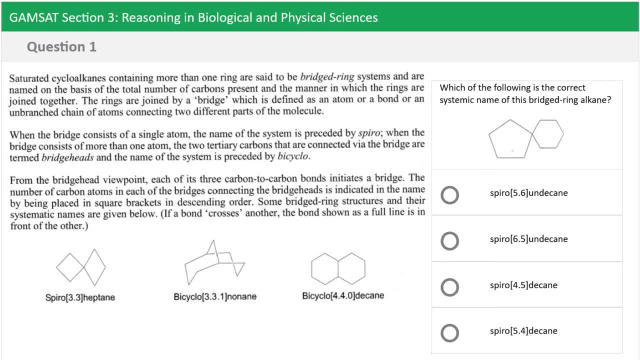 We can actually ignore that. Okay, so the fact that we know that the spiro probably is referring to the fact that it's a two ring structure connected at one point, that's enough for us to move on and see what else we can have a look at Now, another thing that we could look at as well: 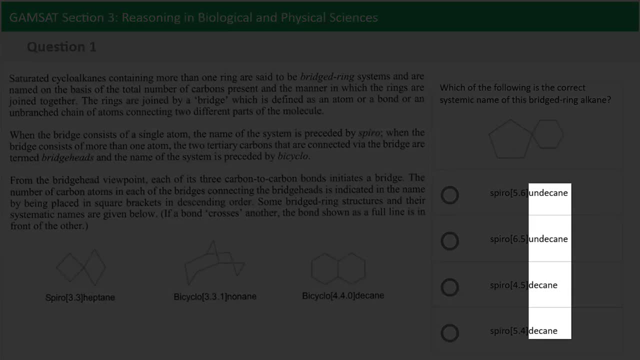 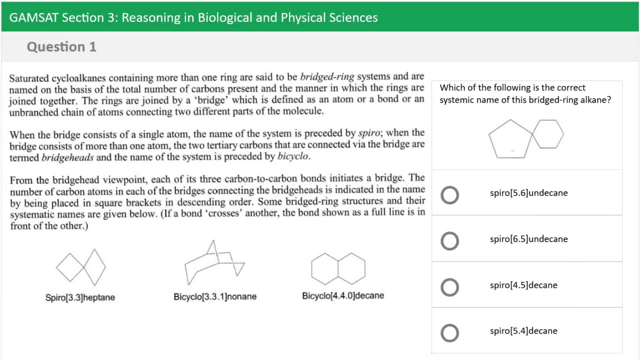 is the end of the name, which is- and I can see that there are two options: There's andecane and there's decane- And perhaps we can figure out what would be the difference between the two. Now, if you already have some familiarity with IUPAC naming, even very, very 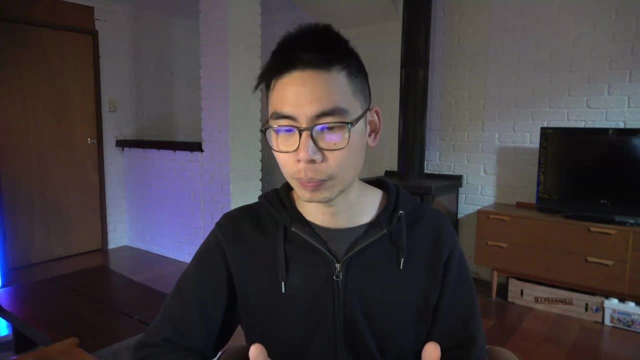 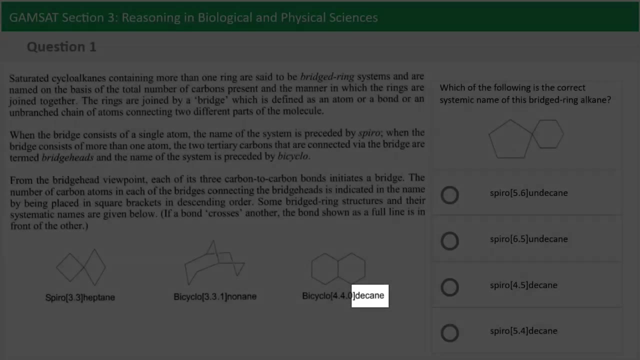 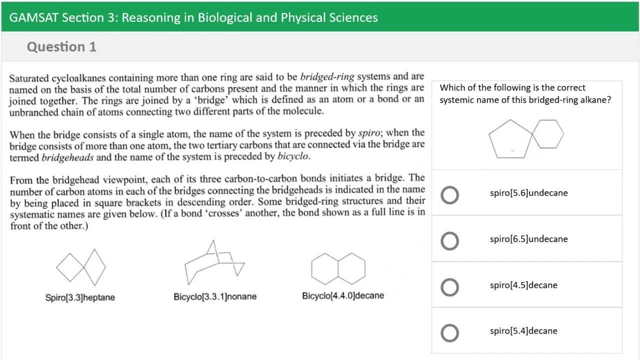 basic. you'll probably recognize decane. Okay, and even if you didn't, we can see that there's an example provided And the prefixes of dec and also andec are referring to the number of carbons And we can kind of check this. In fact, you can see why they're. 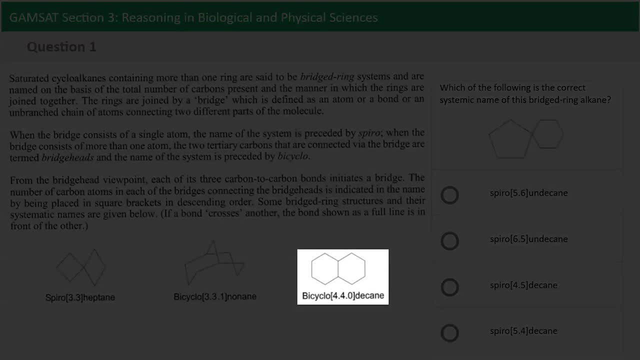 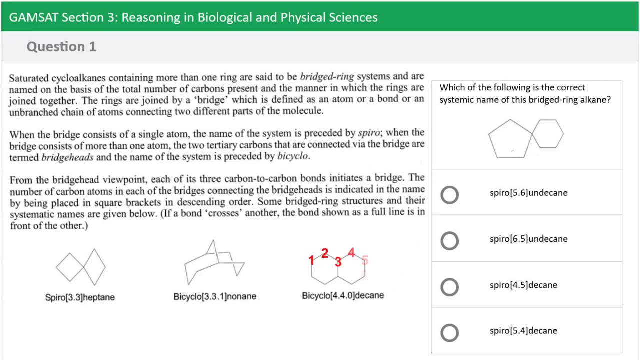 giving us this example, Because if we looked at the last molecule that's provided in the example, which is called bicyclo 440 decane, if we check the number of carbons in this molecule, it is 10.. And if we check our molecule and count it, it is also 10.. So what this tells us is: it's highly 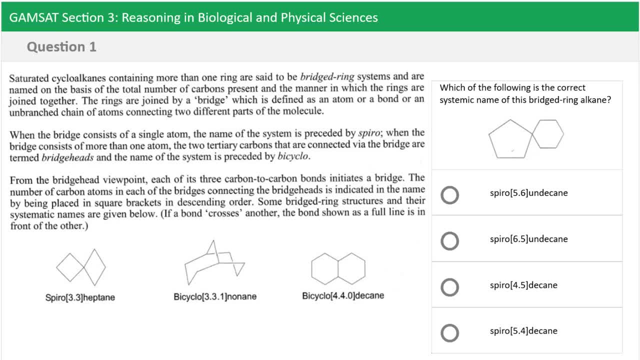 likely that our molecule is also a decane. This means that we can already eliminate half of the options. The only real difference between the remaining two options now is whether or not it's 4, 5, 4, 5, 4,, which is the order of the numbers in the brackets. 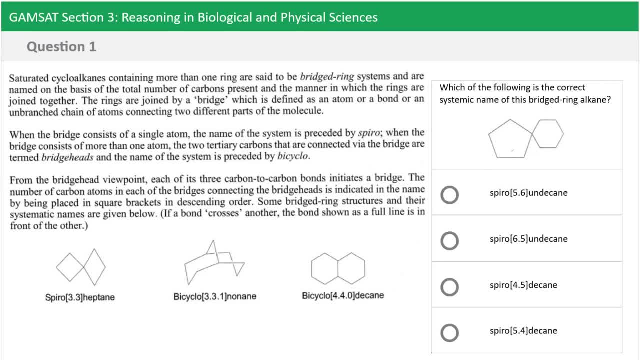 So if we make that our goal, like to figure out which order should it be, and we have a look at the text, we can see- and I'm skimming the text now so I can see- that there's references to numbering in the third paragraph. So here let's have a read. 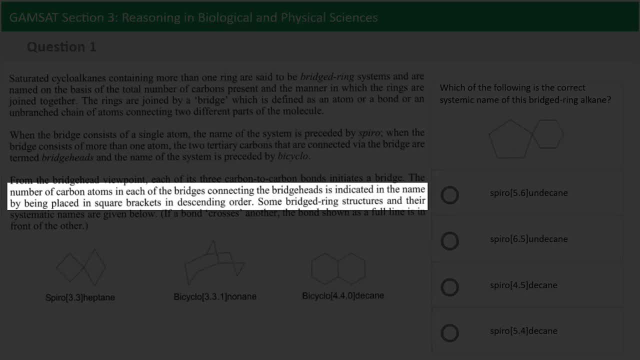 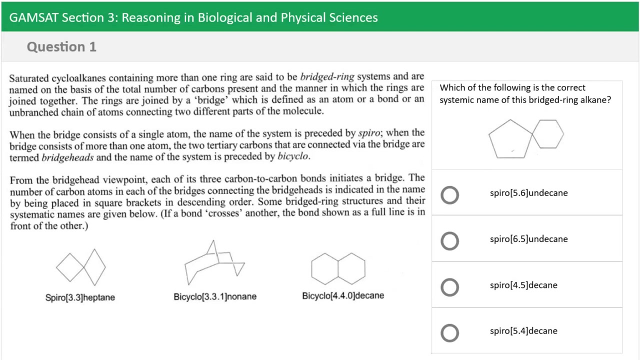 The number of carbon atoms in each of the bridges connected the bridgeheads is indicated in the name in the square brackets. there we go. So that's referencing to the numbering system in the square brackets, And if we keep on going in descending order, okay, which means that we 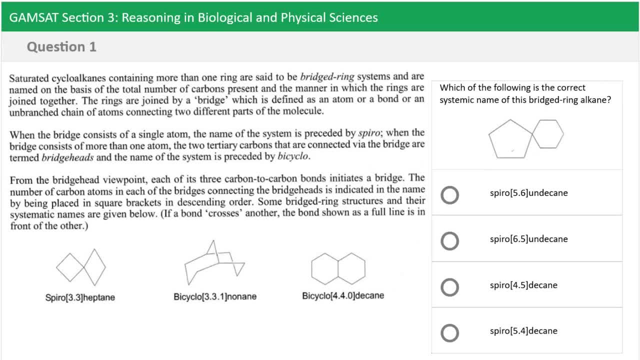 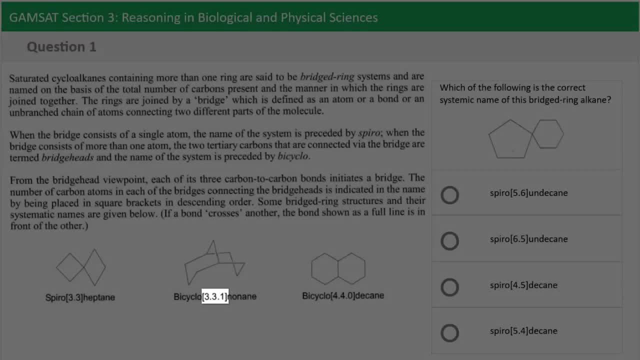 have to place the numbers from largest to smallest, And we can see from the examples that indeed, that's what happens when we look at, for example, bicyclo 3- 3, 1 non-n and bicyclo 4- 4- 0,. 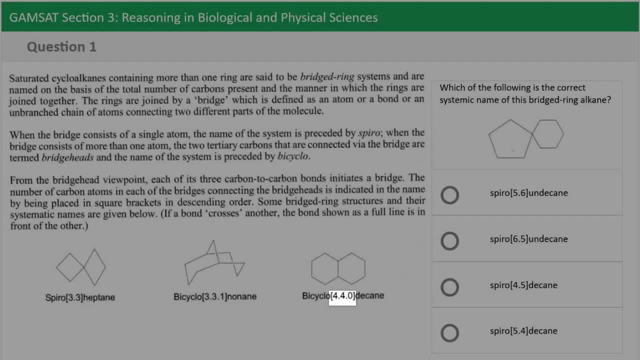 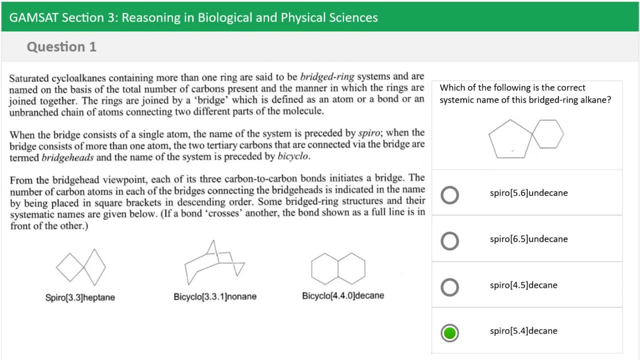 we start off with the larger numbers first and we end up with the smaller numbers, So that means the answer should be spiro 5, 4, decane, because it's in descending. the numbers are in descending order, So I hope you can see that we didn't need to use.